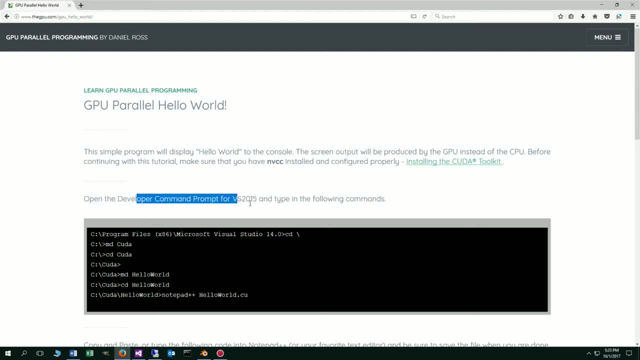 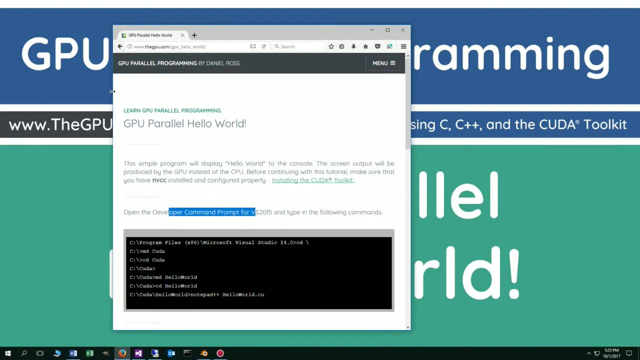 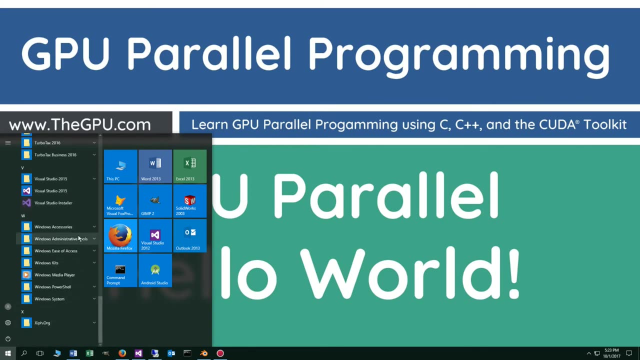 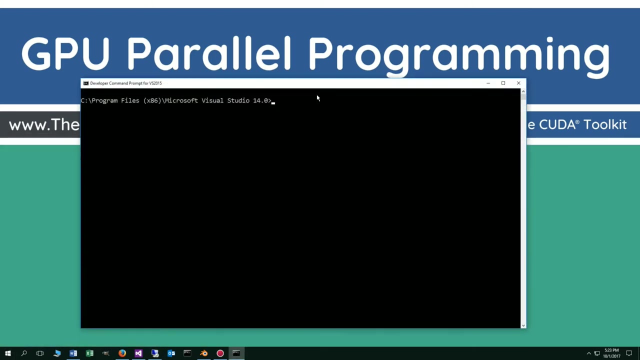 Okay, so what we're going to do is open the developer command prompt for Visual Studio 2015.. I'm going to go ahead and move this off screen here And let's go back Scroll down here: Visual Studio 2015.. Developer command prompt for Visual Studio 2015.. Not just any command prompt there. 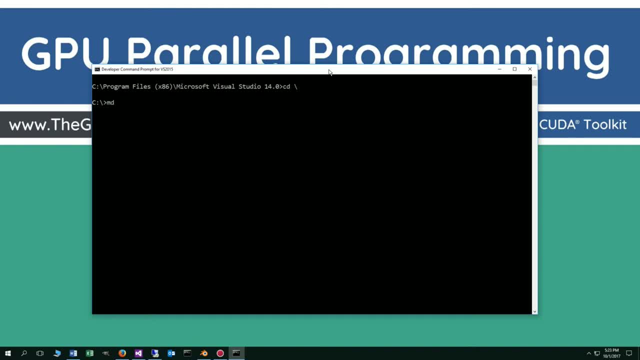 Okay, we'll do cd backslash. It takes us to the root. make directory CUDA. I already have that subdirectory, but if you don't, I'm going to create it for you. I'll change directories to the CUDA subfolder and make a directory here called Hello World. 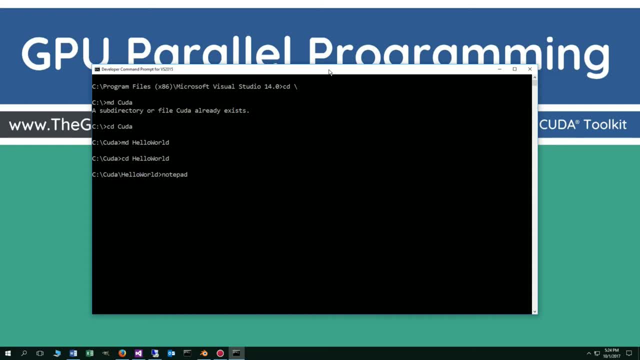 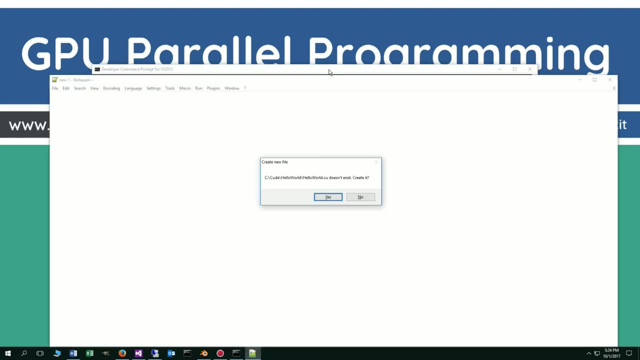 Okay, I'll change directories to the Hello World folder. I'll do a cd backslash Dockerpad++helloworldcu for the CUDA program there. Proper extension. We're going to create it. yes, Alright, let's come back over here to my website. 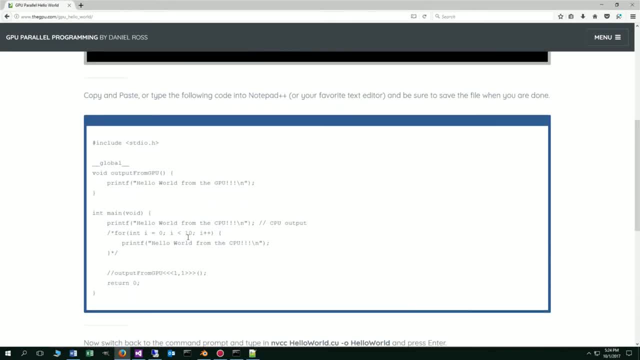 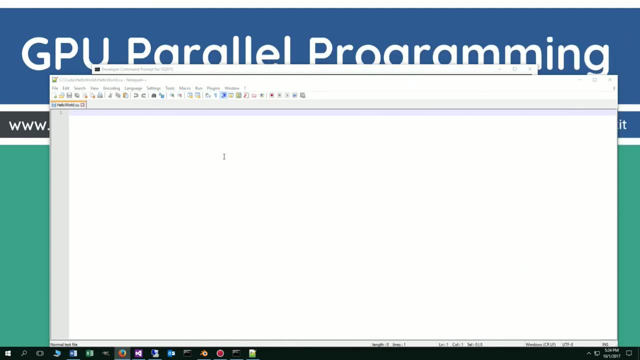 Here's where we're at right now, And let's grab all the source code here. You don't want to see me type this in there, so we'll just go ahead and copy that and paste it over here. Okay, now I'm going to come up here and save this now. 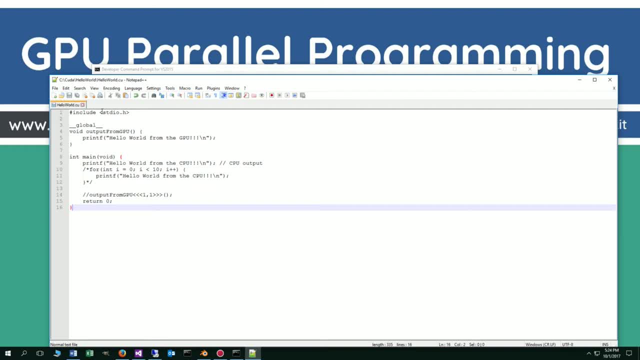 Okay, now I'm going to come up here and save this now. Okay, now I'm going to come up here and save this. now up here and save this and talk just briefly about a couple of things here. pretty standard there, no need to talk about that. here's our main function here right now: what this is going to do. 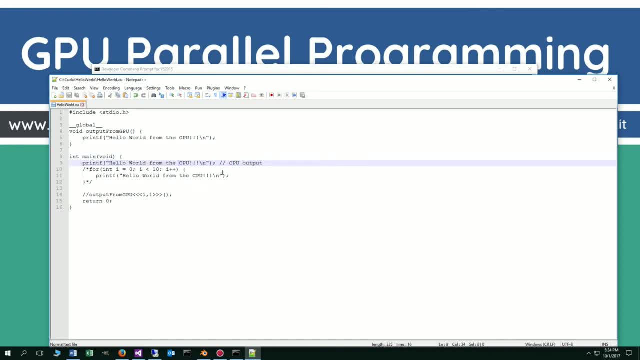 we're just going to do a simple printf: hello world from the cpu. this is all pretty standard here- and then i've got a for loop world display at 10 times to the console, and then i've got this new line down here and ignore what this is up here for the moment there. so what my strategy here is? i'm just 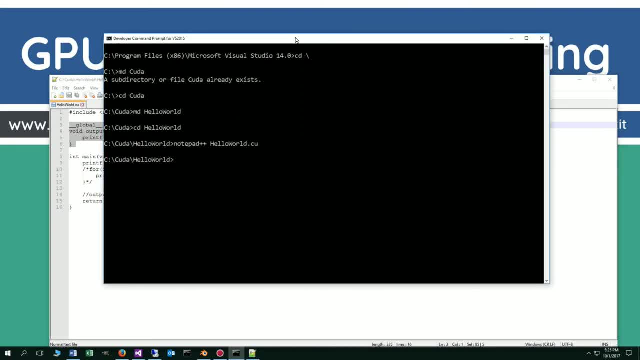 going to talk about normal. you know, straight line by line execution, serial execution, basically in a cpu there, not parallel- and then i'll show you how to do stuff- the same thing with parallel and how that works. so what we'll do first is do an mvcc and i'm going to take this as in, really like baby. 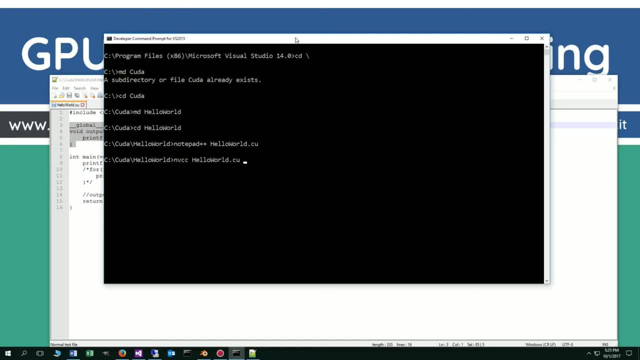 steps as far as this is concerned here initially there and our output file, we'll just do hello world. okay, we've got our hello world exe. we also have this exp file and a live file here and i'll go in future tutorials i'll go what those are there. so, uh, just executing hello world, exactly what we. 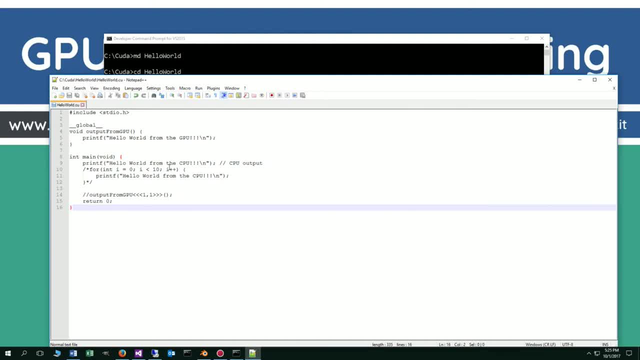 would expect hello world from the cpu with a new line escape sequence there. all right. now let's say, for example, in a cpu type program, a serial program, there we want to display um you, hello world 10 times. right, we have to go through a simple basic for loop. you know other ways of. 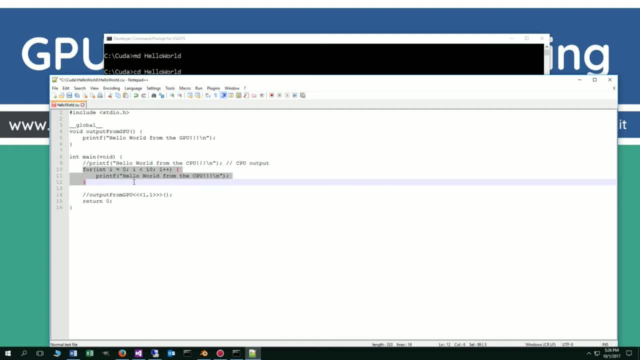 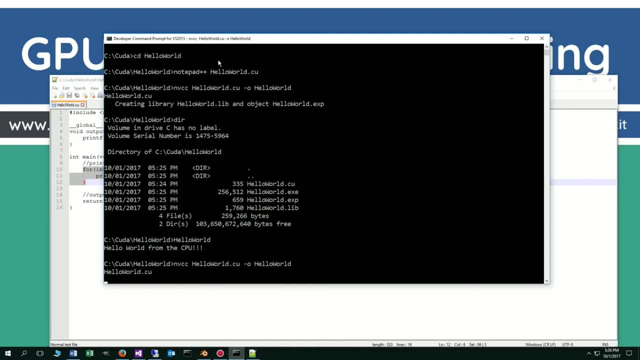 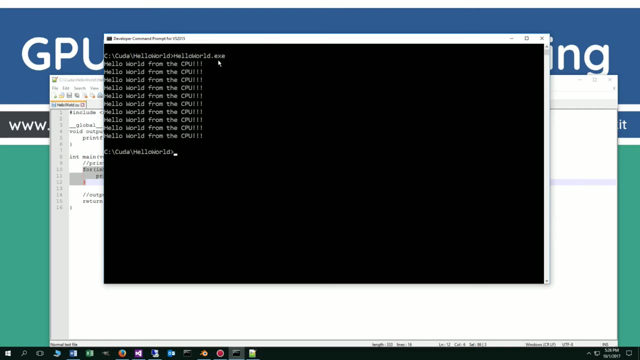 doing it, but for loops, by far the most common way. hello world from the cpu. all fairly simple there. just bear with me and we'll just recompile this again, rerun it and we'll go ahead and clear off my screen here and we'll just do the hello world exe and we've got it displayed 10 times to the 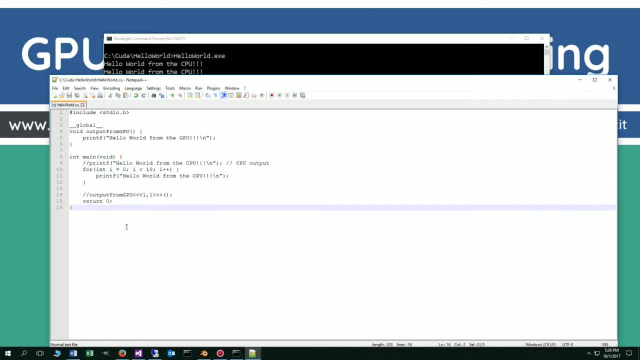 console. all right. so what we're trying to do basically with this is we're going to do a parallel programming as we're trying to tap into the power of the gpu with all of its parallel processors and parallel threads, okay, and we define a parallel function right up here using this. this: 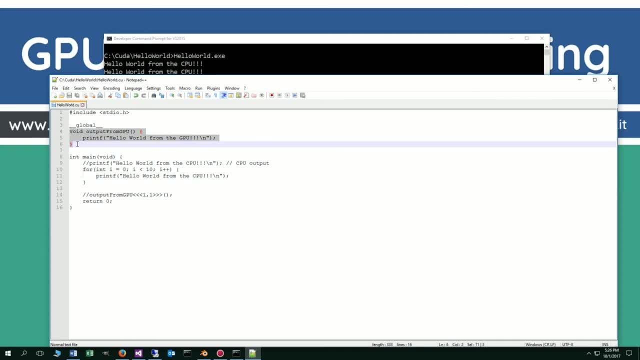 global tag right here. and then this looks like an ordinary c function, but it's in the world of gpu programming. it's called a kernel, k-e-r-n-e-l, right. and so this whole entire thing here, what looks like a, you know, a function here is basically called a kernel and we're going to do a parallel programming. 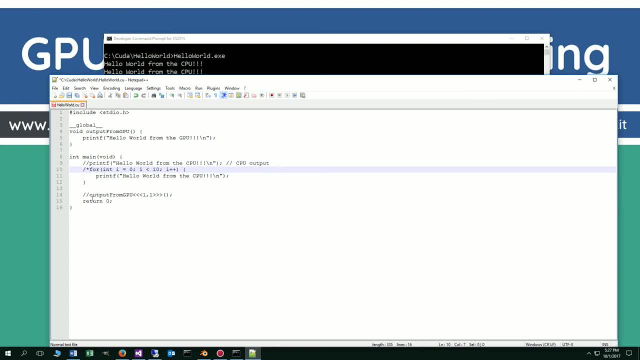 of the kernel. i'm not going to get too in depth into this hello world here, but we'll go ahead and comment this out, right, and if we come down here and uncomment this line of code here, i'm just going to save this real quick. here it. it looks like we're just basically executing, calling, or. 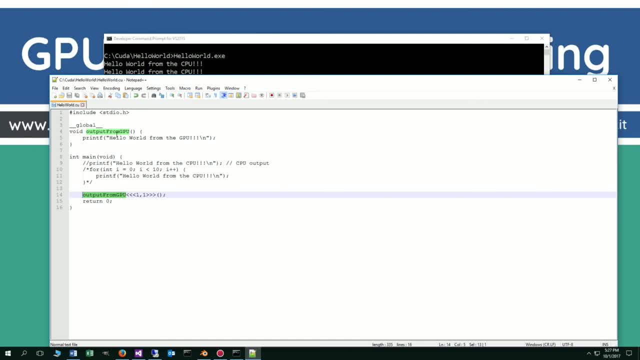 invoking whatever terminology you prefer, this output from gpu kernel right, function per se, without this funky looking syntax in between the the name of the function: right. this makes it a kernel okay. now you get these triple chevrons open and closing there, and then you've got basically two parameters that we're going to talk about initially here. 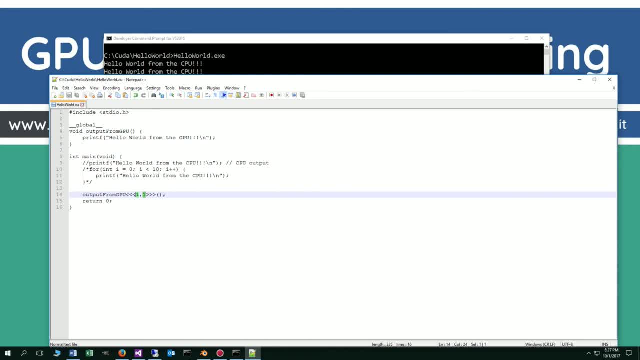 and i'll get into this a little bit more in future videos. these are actually a lot more. there's a lot more to them than what you're seeing right here. but basically we're telling it: we're going to execute one thread on one block. okay, so let's go ahead and compile that and see what happens there. 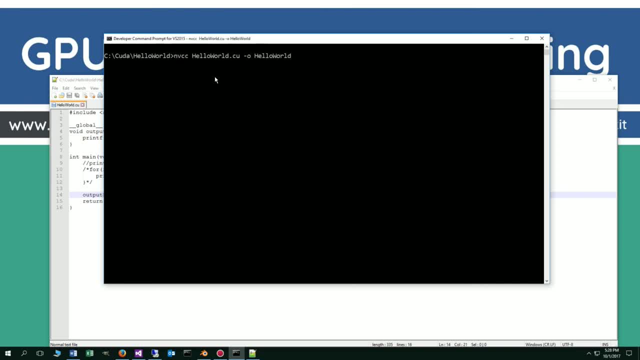 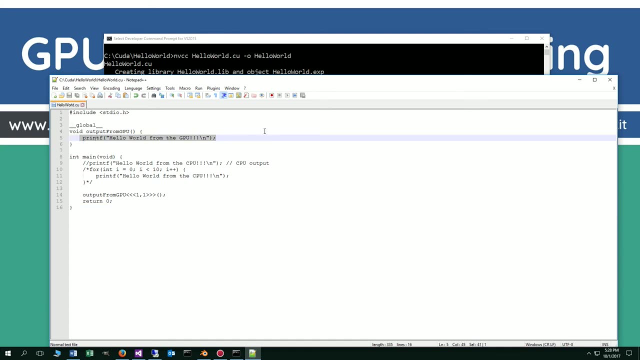 okay, clear our screen, compile and run, and there we go. we got hello world from the gpu. now, technically, at this point in time, you can see that, uh, you got what's called host and device. uh, hosts and devices. right, the host is the cpu and the device is the gpu. so the gpu actually executed this code here, but we called it from. 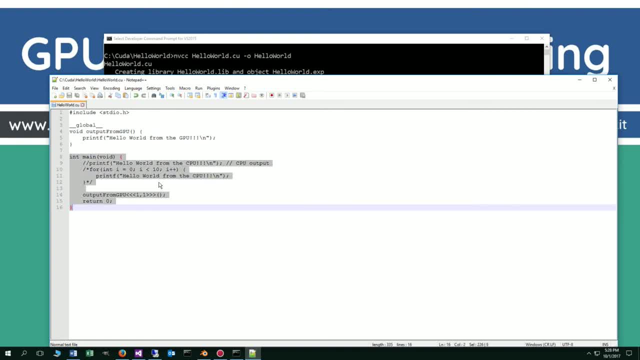 within the host device, because in the main this is just the standard main function here. the cpu called this all right. so let's say, for example, we want to do the exact same thing as this for loop up here. so we're going to do, we're going to. 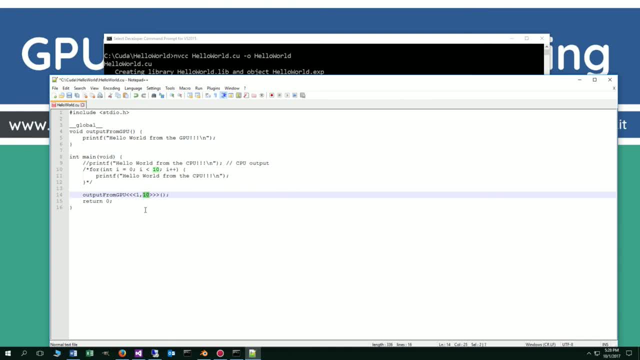 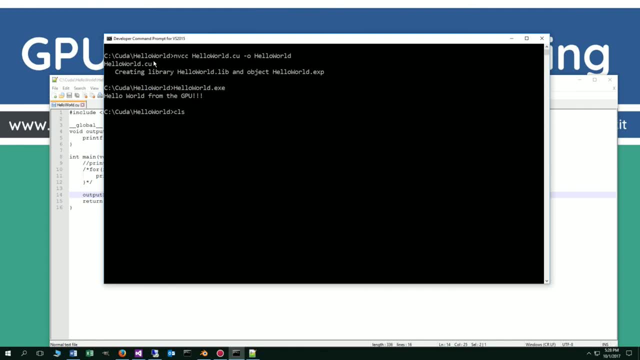 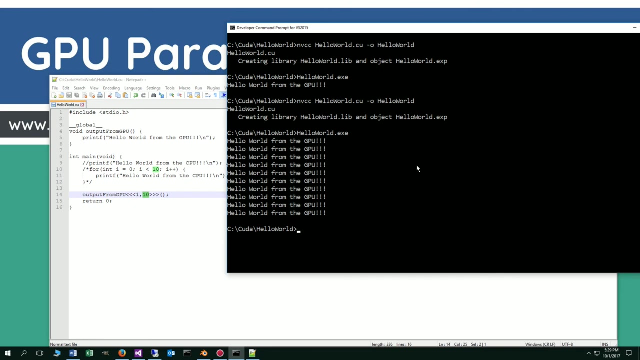 do one block, but we're going to do 10 threads, which will execute 10 threads simultaneously here on this. okay, let's go ahead and save this, recompile this and rerun it there. okay, and now, as you can see, we have got hello world from the gpu executed 10 times and there's no loop or anything like that. we'll just 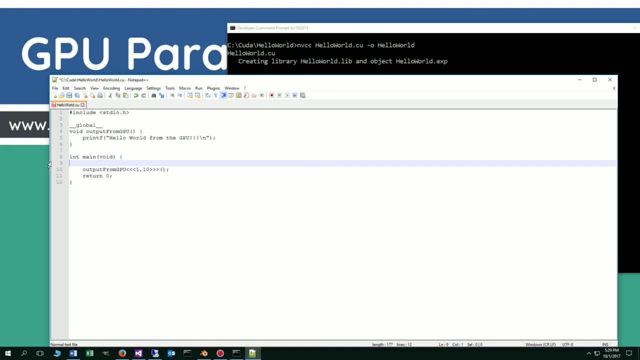 take out all of the all of the cpu stuff that i threw in there, and this is as simple as the program gets right here if we want to display this. so let's say 1k time 1024 there to the console, let's go ahead and save it there. this will open up 1024 threads. each one of these threads will display this. 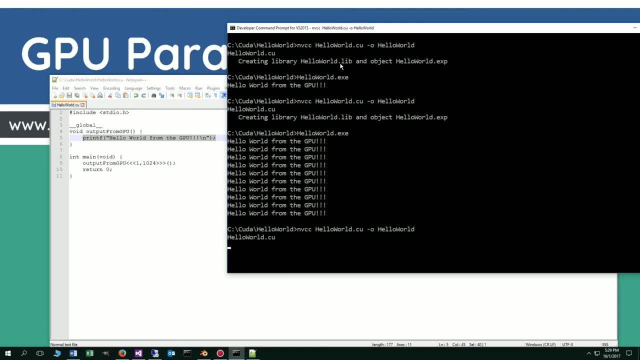 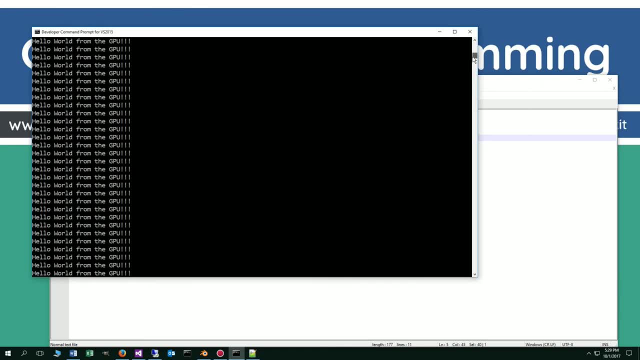 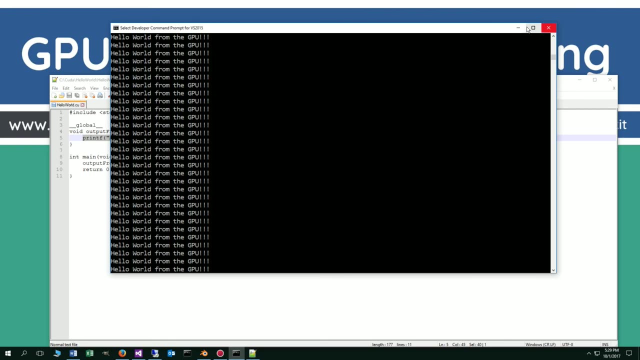 to the console there. all right, and um, i don't know about me run that and there we go. we've got 1024 threads on the gpu all displaying hello world from the gpu. all right, um, as far as this tutorial goes, i think i'm gonna go ahead and 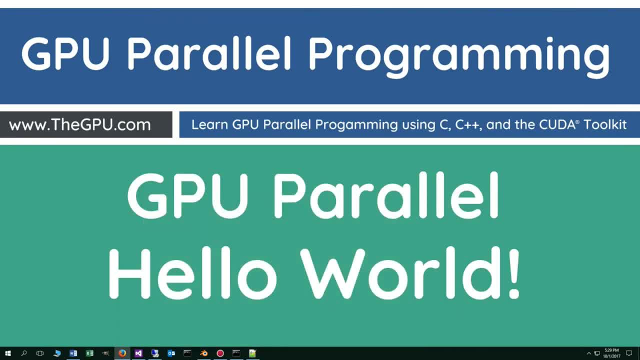 just uh close out that, close out of that and uh leave you guys with some, some simple thoughts or some final thoughts here. so you know, don't worry if the code doesn't make much sense, complete sense yet. i've got a lot to go over with. but um, and i'll d, i'll go over a detail in future tutorials, but the 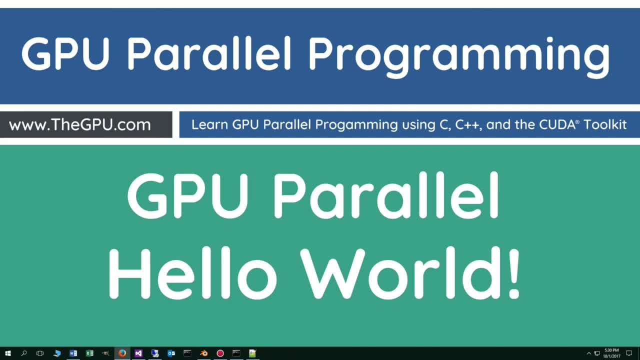 primary goal of this tutorial is to make sure that i've got a lot of code that i can use to run this. so i'm going to go ahead and close out that. and i'm going to go ahead and close out this tutorial was just to give you a little taste of how a cuda program, parallel program, is structured. so anyway, uh, that concludes this tutorial. thanks for watching. 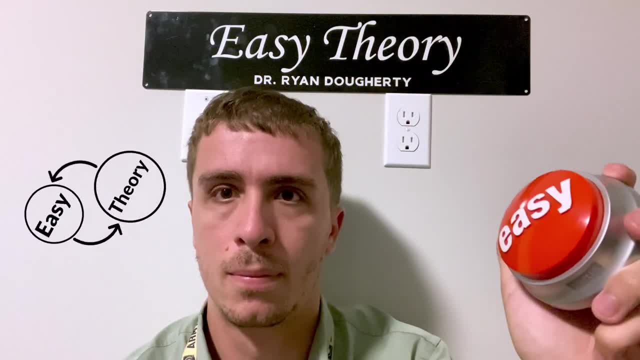 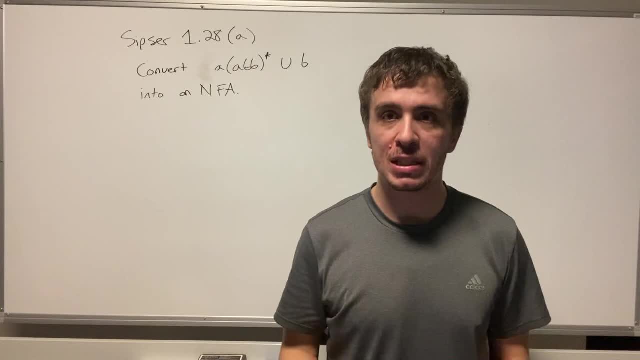 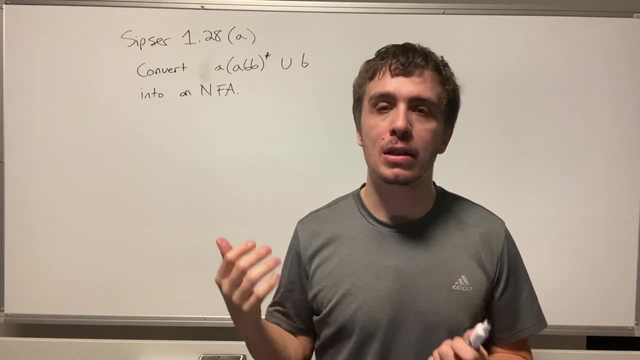 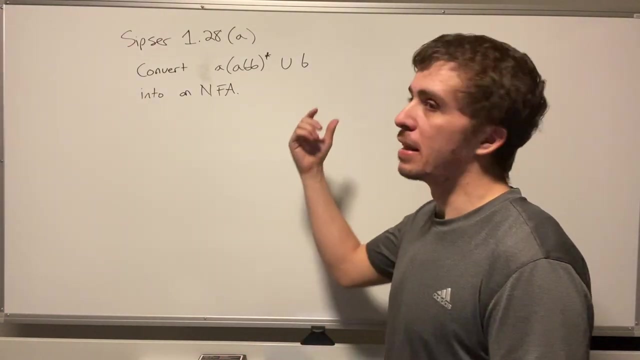 That was easy, All right. so we're going to be learning about NFAs, regexes and how to convert this particular regex into an NFA. So the general strategy here is that you want to start with the really easy pieces and then build them up from there, And by easy pieces I mean the things that 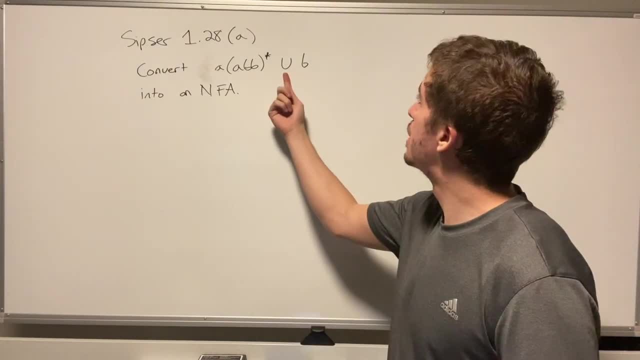 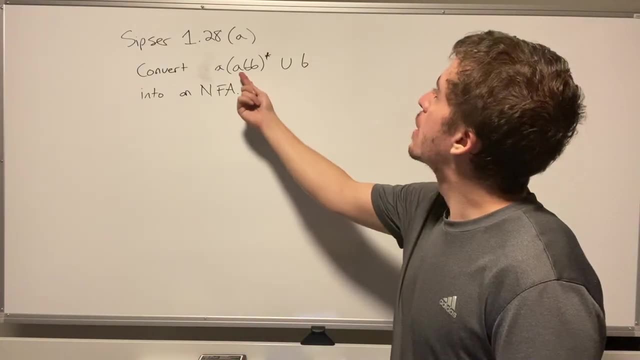 can't be subdivided into smaller parts. So if we look at this union, for example, it's the union of two things, and so therefore can be broken into smaller parts. If we look at each of these individual characters, well, in here too there's going to be concatenation of things, and so those 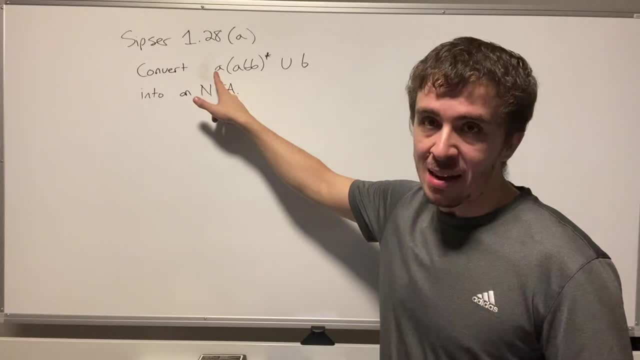 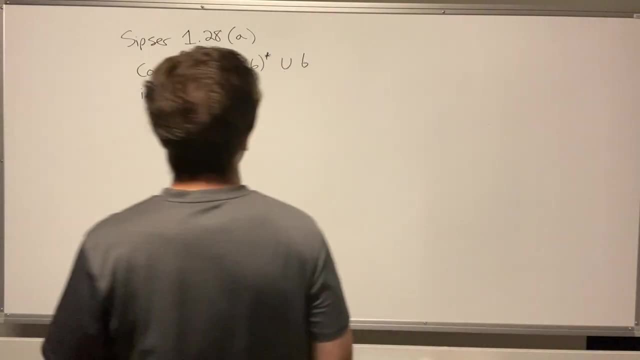 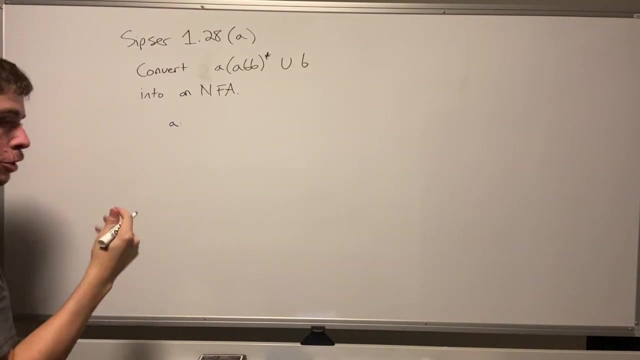 can be broken into smaller parts. But if we look at just the A or just the B, then those can't be broken down. So the general strategy here is to make a little NFA for each of those pieces. So I'm going to make a little NFA for just the character A. So we want to accept just the. 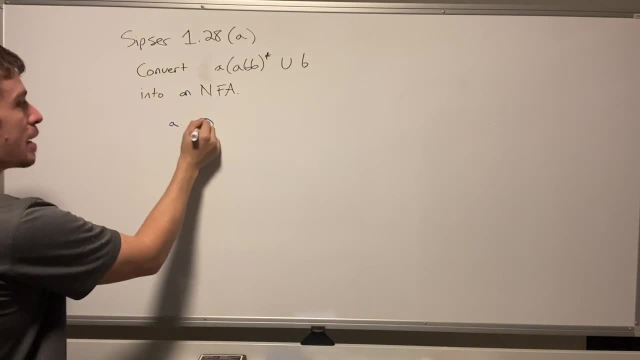 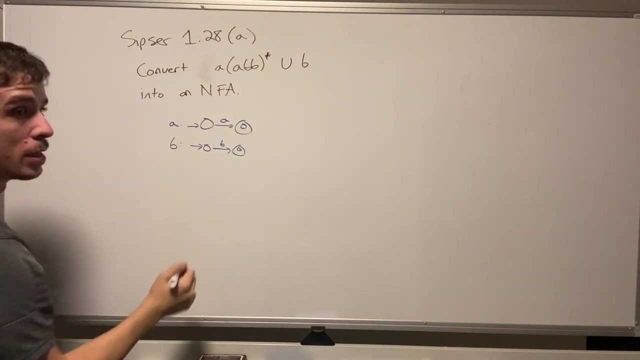 character A and nothing else. And a really easy way of doing that- although there are many- is that I can just have a two-state thing like that, where I just read the A, no other transitions, And then B is going to be very analogous, where I just have a B transition and nothing else. 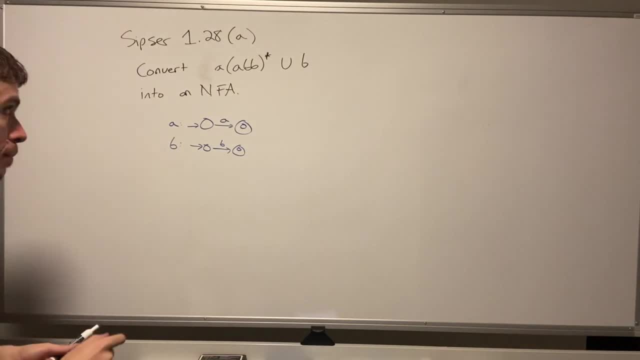 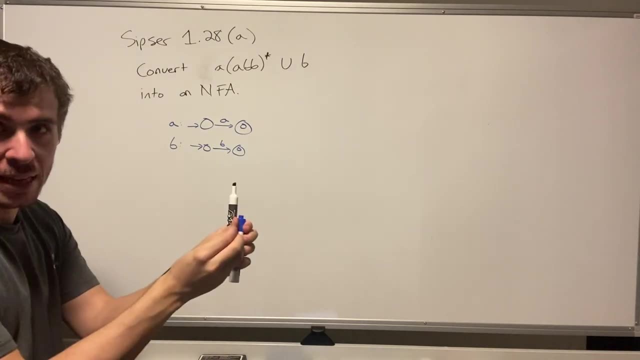 All right. so then what we want to do is we're going to build this thing one layer at a time. It's kind of like an onion, where you start with, like the inner layers and you start building outer and outer layers until you got the whole thing. So what we